And here's what I'm going to do: I'm going to break this apart again. So what I'm going to do is I'm going to break this apart again. The cube root of 3y over the cube root of 2.. And here's what I'm going to do. I'm going to break this apart again: The cube root of 3y over the cube root of 2.. And here's what I'm going to do: I'm going to break this apart again: The cube root of 3y over the cube root of 2.. 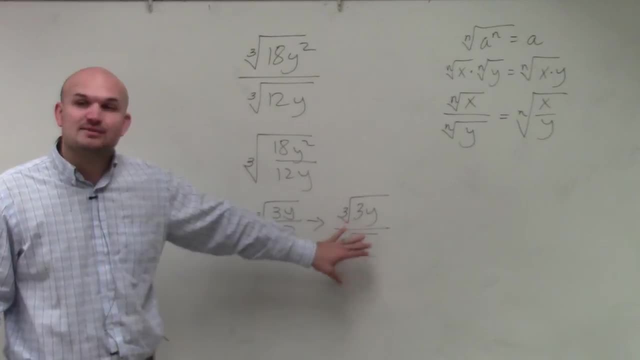 Now, if you look at that, You're just going to have to read the directions. A lot of times there's nothing really wrong with this, but a lot of times they say it's not simplified unless the denominator is what we call rationalized. 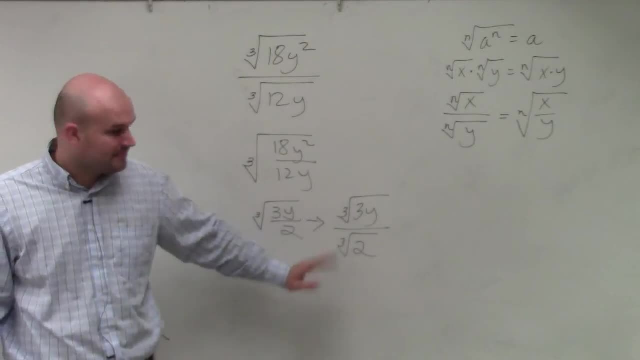 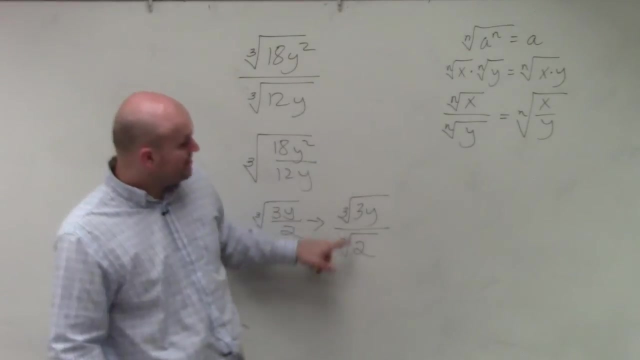 Meaning: you cannot represent a radical in the denominator. So what you do in this case is: if we're looking at this, we need to get rid of the cube root of 2.. Now, to simplify this, I can only take the cube root of 2 raised. to what power? 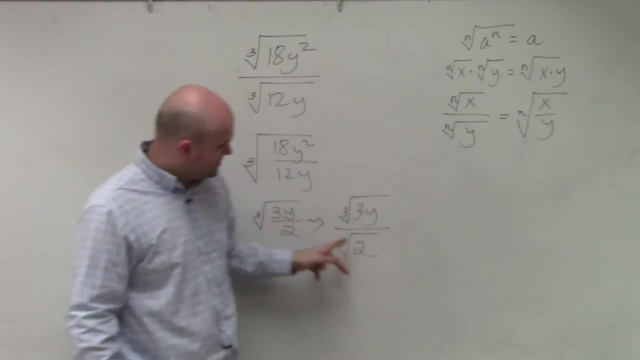 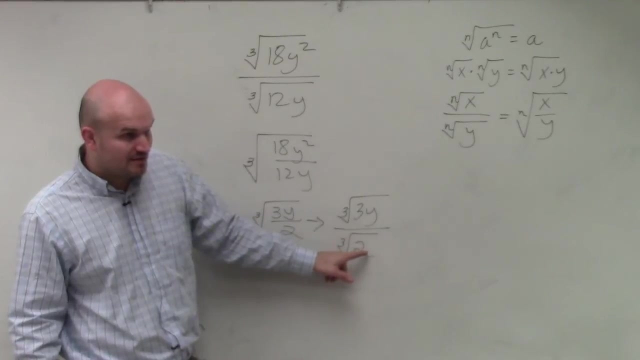 Well, what does this? what power does this 2 need to be so I can take the cube root of it? 3r, 3, right. What power is my 2 being raised to? right now It's 1.. 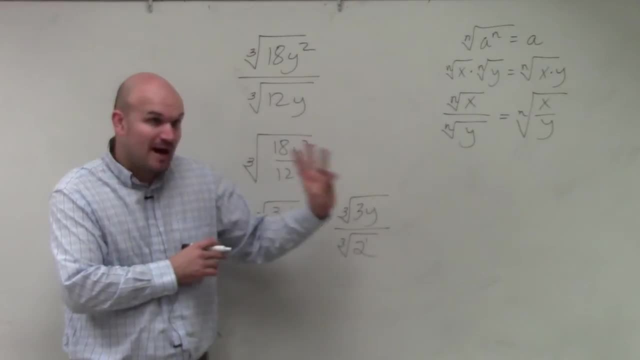 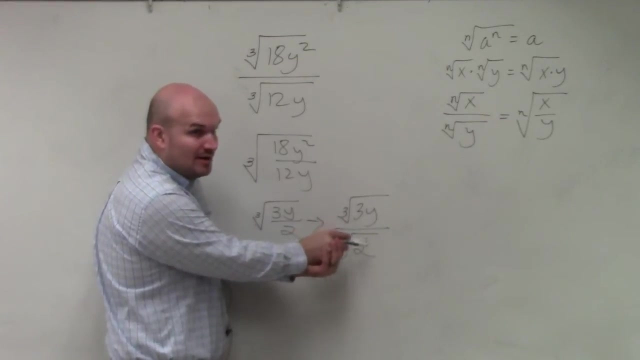 I need this 2 to be raised to the third power. right 2 is being raised to the first power. I can't take the cube root of 2 to the first power. I can only take the cube root of 2 to the third power. 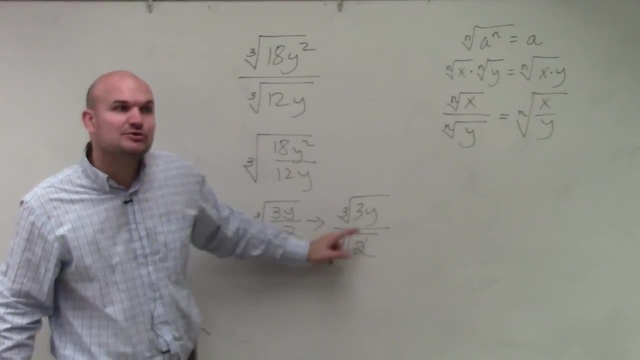 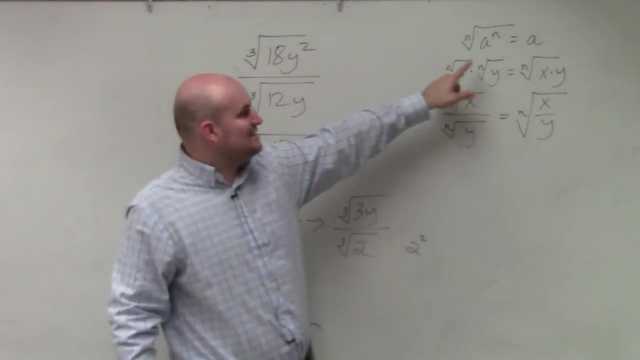 So why do I need to multiply 2 to the first by to get it to be 2 cubed 2 to the second power? However, is there any rule up here that says you can take a number outside of a radical and multiply it to a number inside of a radical? 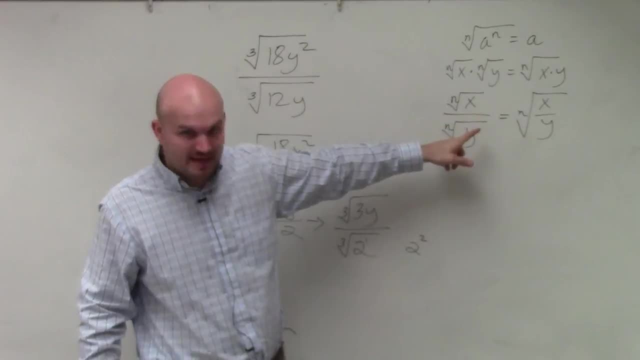 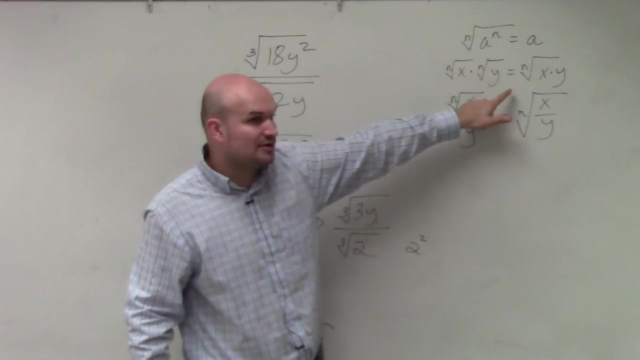 No, there's nothing I wrote up there that says that Guess what. You cannot do that. However, there is a rule that says if your indexes are the same, whatever's inside your radical, your radicands, you can multiply. 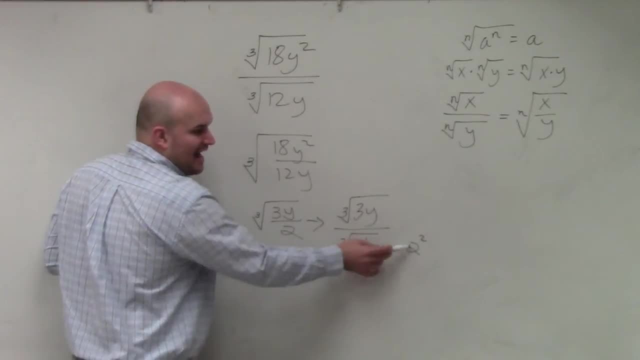 So, therefore, if I want to multiply this times this, I need to make sure these are the same radicals. So therefore, I need to multiply this by By the cube root of 2 squared, And whatever you do in the denominator, you have to do in the numerator. 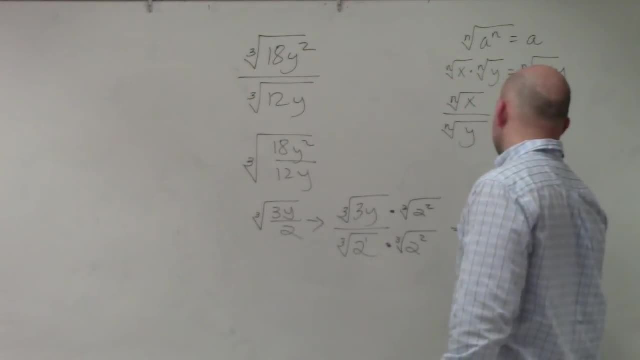 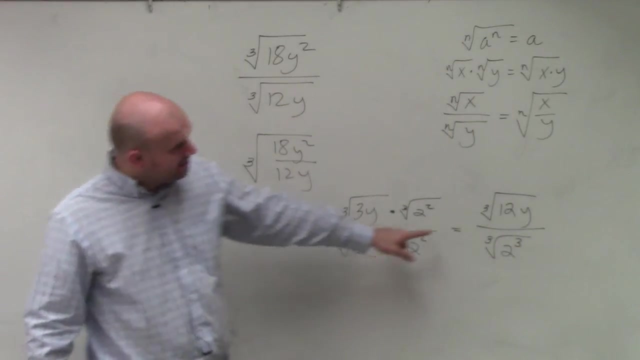 So now, by doing that I get the cube root. Really, 2 squared is 4, correct. So 4 times 3 is 12y Over. this becomes the cube root of 2 cubed. Well, as we've mentioned, the cube root of 2 squared is 4.. The cube root of 2 squared is 4.. The cube root of 2 squared is 4.. And the cube root of 2 squared is 4.. So 4 times 3 is 12y.